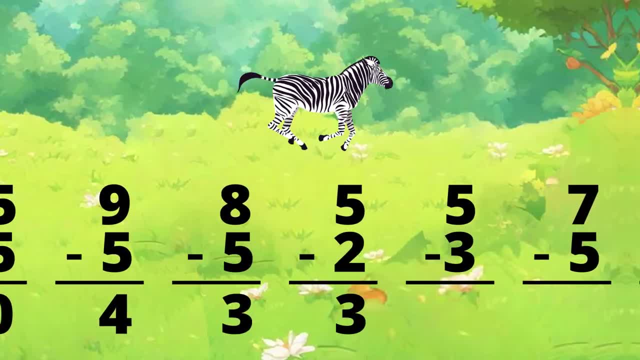 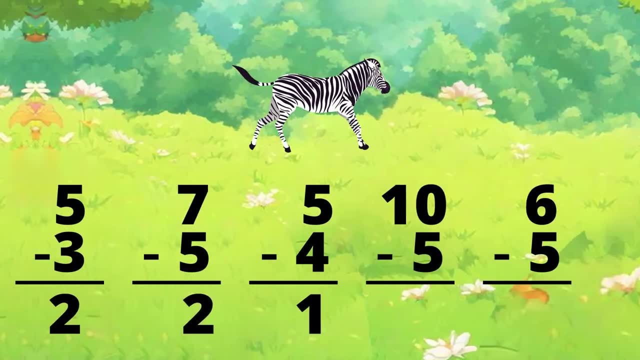 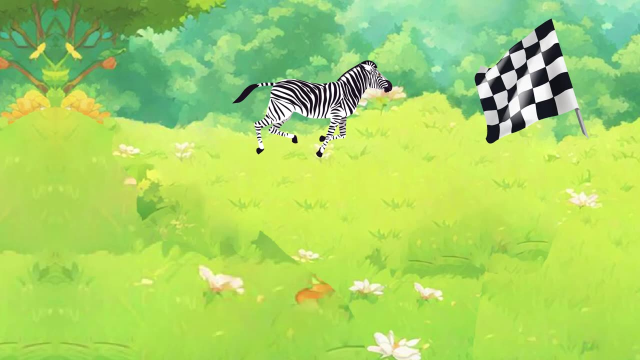 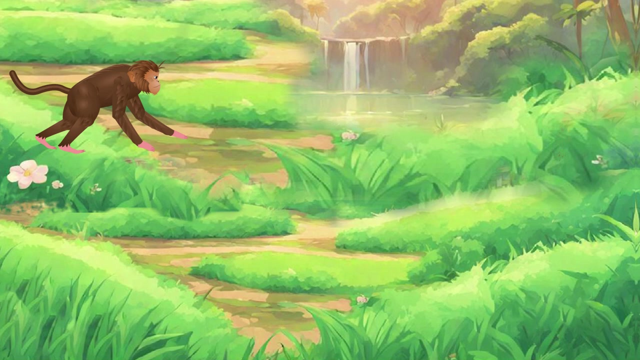 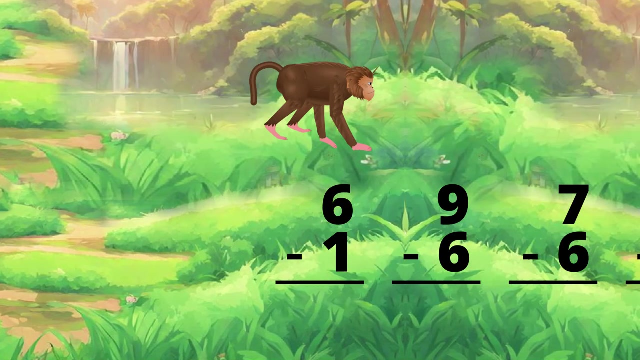 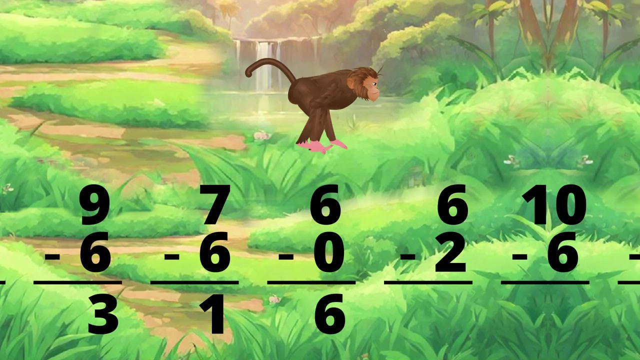 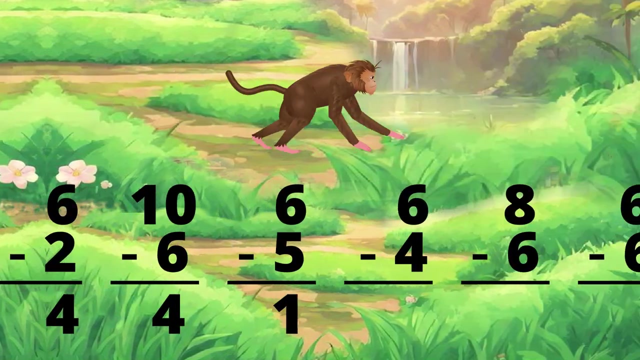 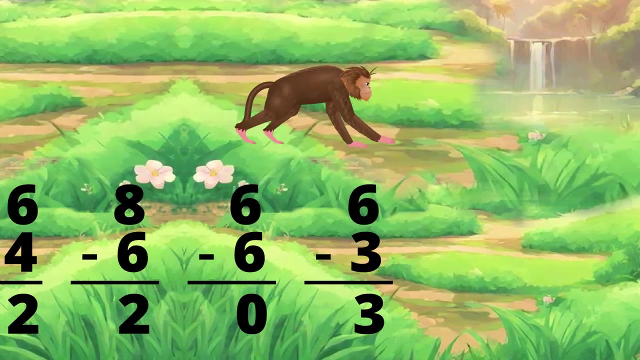 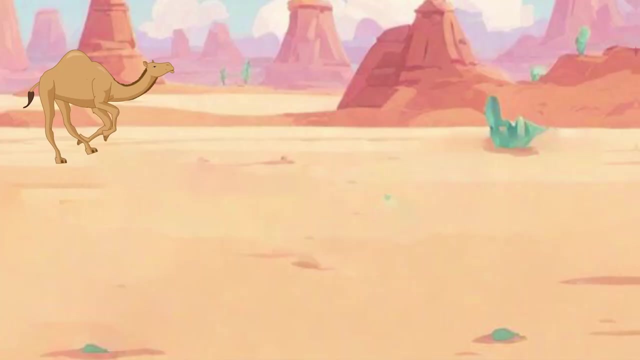 Music, Music, Music, Music, Music. Were you faster than the zebra? This race will test you're knowledge of subtracting six, Competing against the monkey: Ready set, go, Music Go. How did you do Get ready to race against the camel to test your knowledge of subtracting with seven. 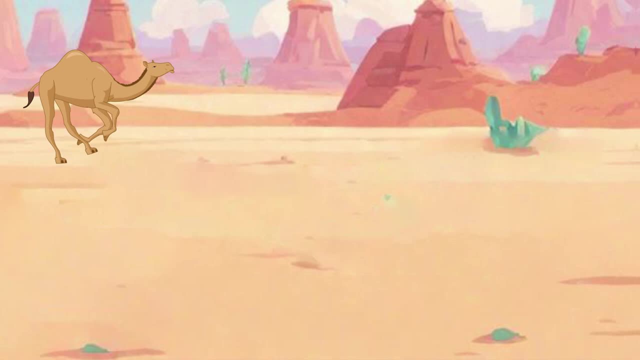 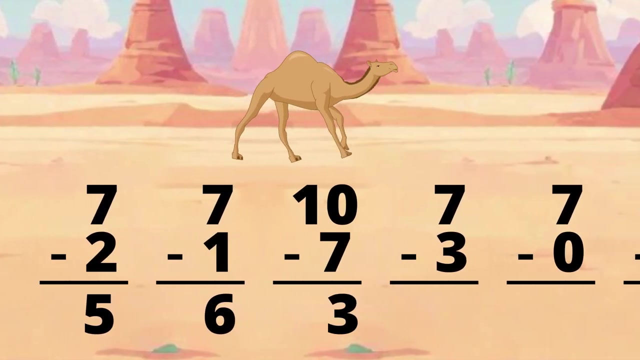 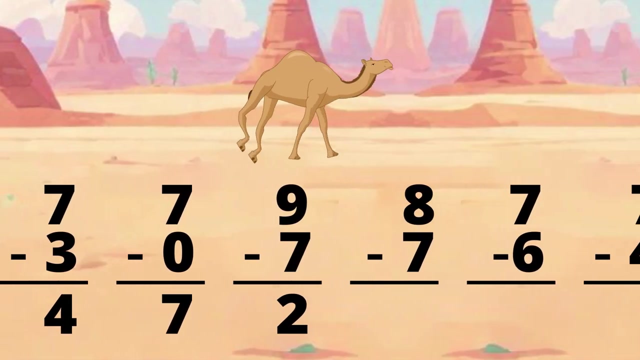 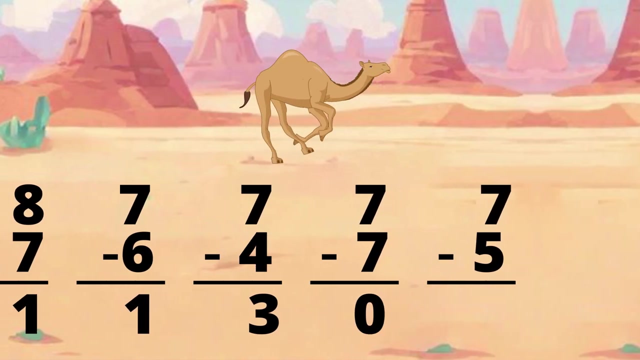 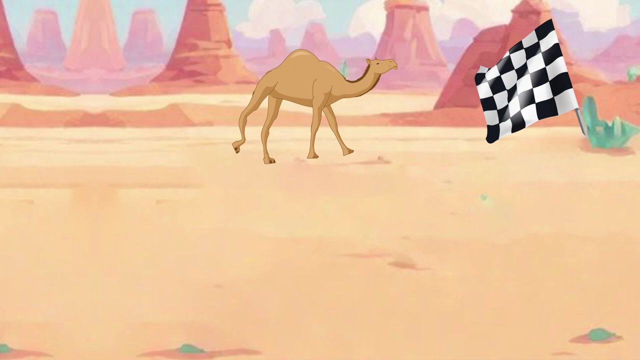 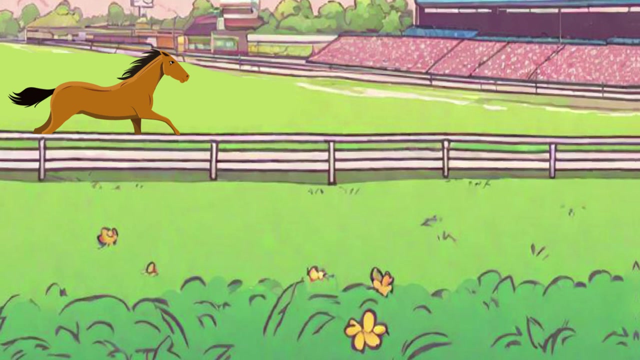 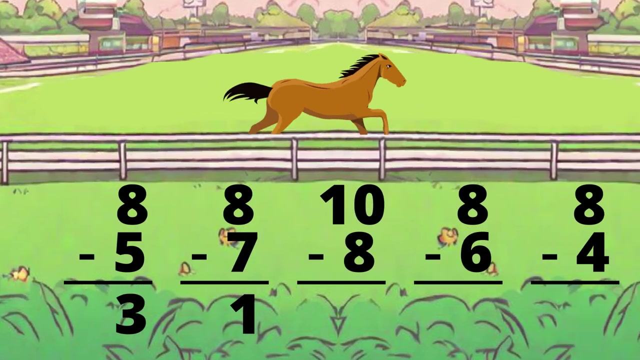 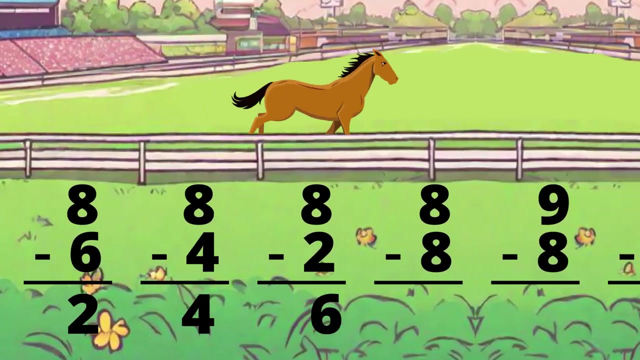 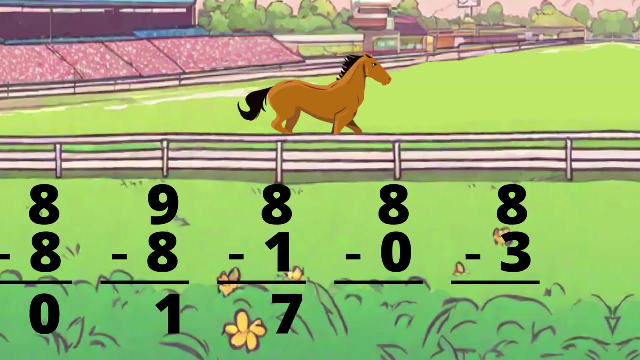 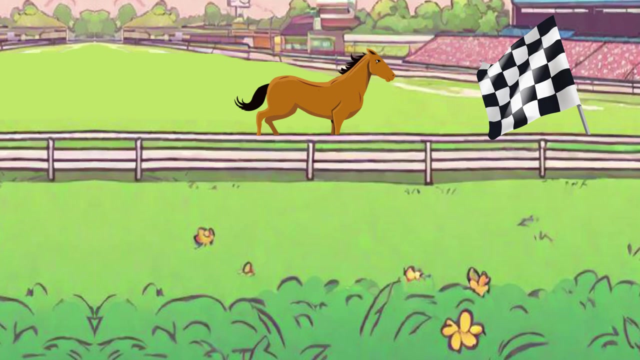 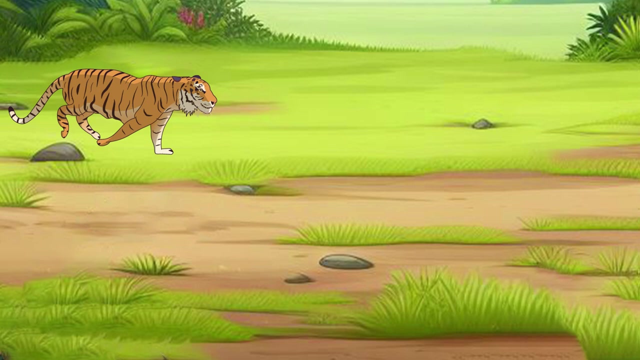 Ready set go. Did you get the answers before the camel did? Now we'll race over the gates with the horse. Ready set go. Were you able to beat the horse? In this next race, you'll compete against the tiger to see how fast you can subtract with nine. 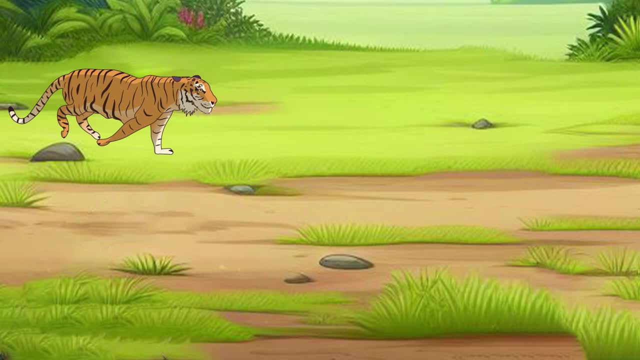 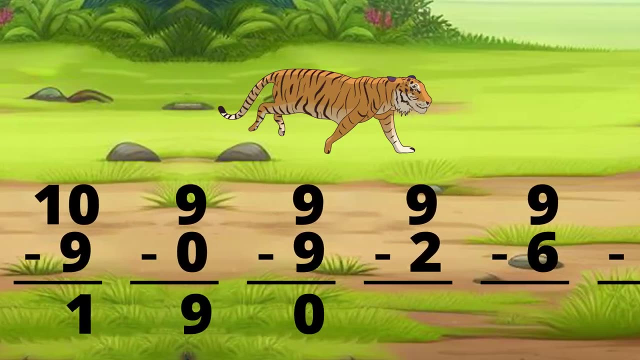 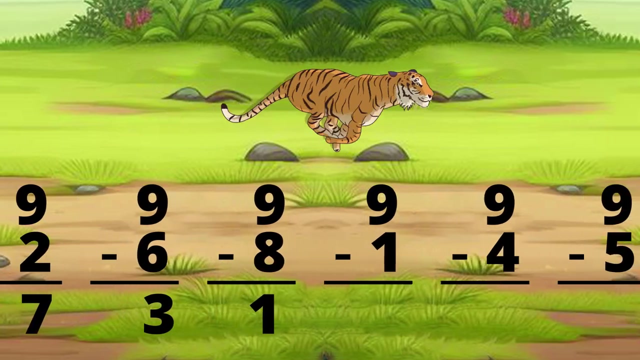 Ready set go. Did you get the answers before the camel? did Ready set go? Were you able to beat the horse? In this next race, you'll compete against the tiger to see how fast you can subtract with nine. 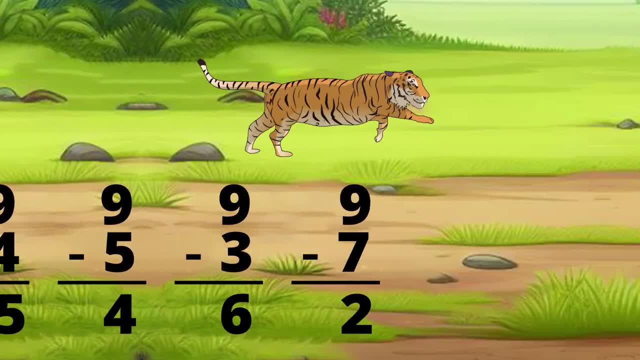 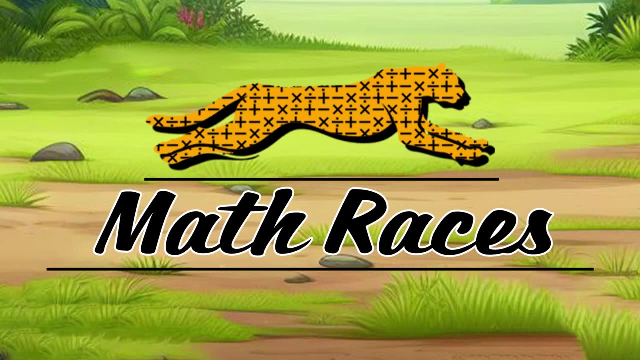 Ready set go. How did you do on your nines? If you didn't do well in some of the races, you can always come back to this video and try doing these math races again.